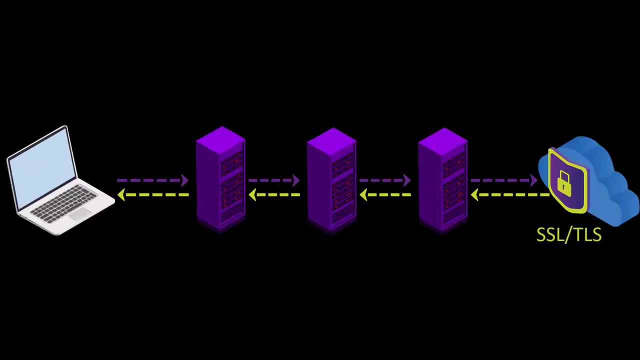 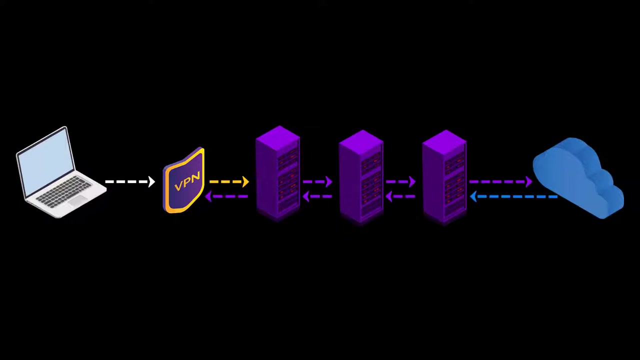 The SSL and TLS certificates mentioned here. both encryption the traffic between you and website. Some the websites use SSL, others use TLS certificate. For the rest of the course, I will be referring the both certificates by simply saying SSL. When you connect to the Tor network over VPN, your internet access appears as like that: 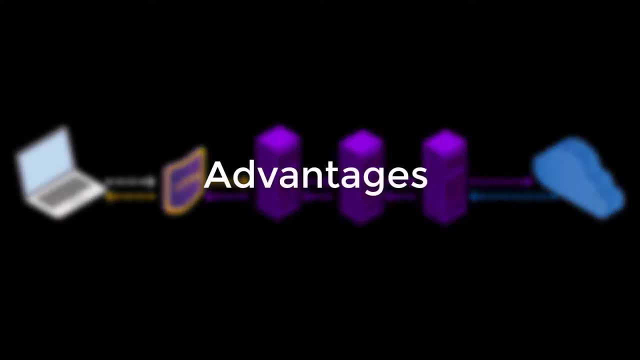 Advantages of connection to the Tor network. 1. Connecting to the Tor network over VPN. Your internet service provider or any observer on your network can't see that you are connecting to the Tor network. It only sees that you have established a VPN connection. Since VPN use is much more common than the Tor network, this creates relatively little doubt about your internet traffic, Because the communication between you and the entry nodes will be encrypted by the VPN. 2. Observer's or malicious entry nodes on the network cannot breach your privacy. 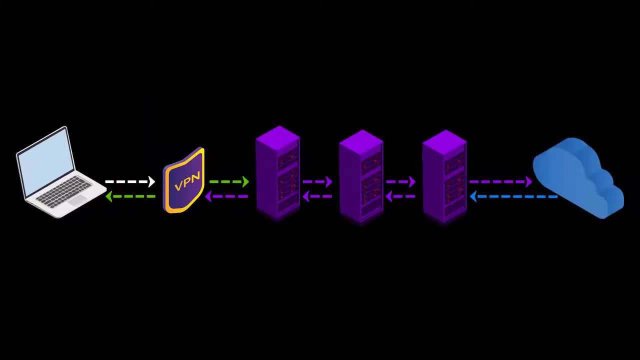 Since the Tor entry nodes will see the IP addresses of the VPN servers you are using instead of your real IP address. you will hide your real IP addresses even if the entry node is malicious. However, for real anonymity at this point, your VPN servers shouldn't be keep logged. 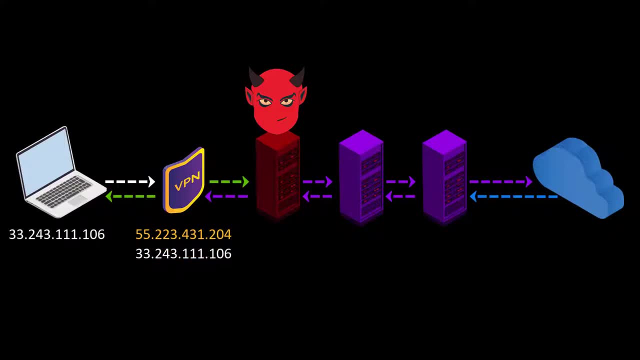 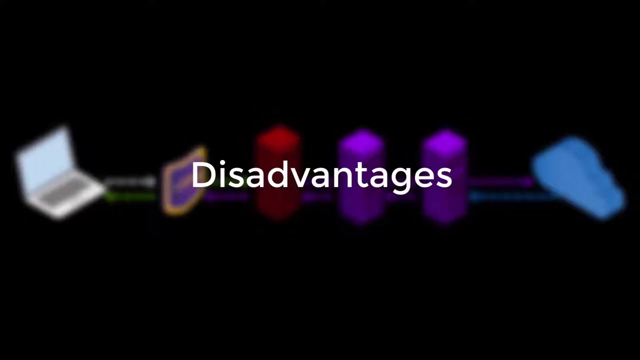 Otherwise, your anonymity may be violated. 3. Connecting to the Tor network over VPN: Your VPN servers know your real IP address. In addition to these advantageous features, there are also disadvantages we experience. when connecting to the Tor network over VPN, Your VPN servers know your real IP address. 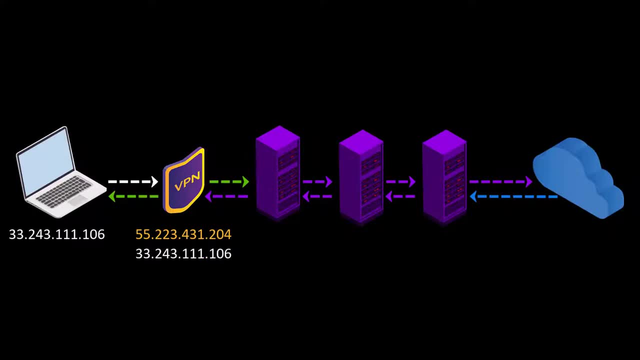 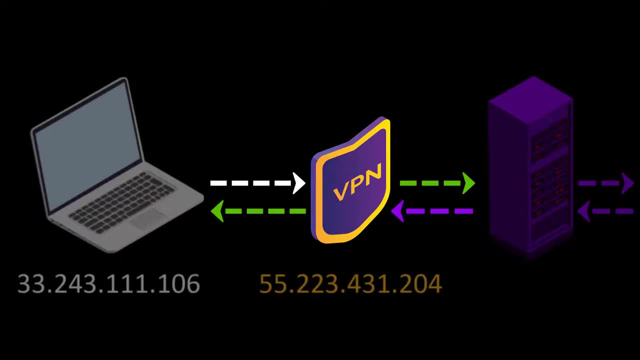 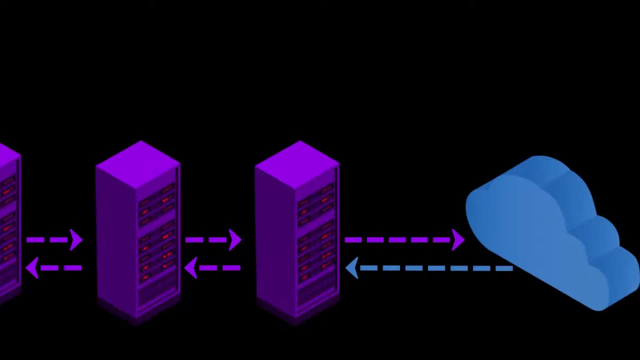 Because VPN only encrypts the data sent from to you, the entry node. the data sent by websites cannot be encrypted by the VPN while reaching the exit node. In such a case, if the exit node is malicious, it may violate your privacy by reading the response sent from the website. However, this applies to any site that doesn't. 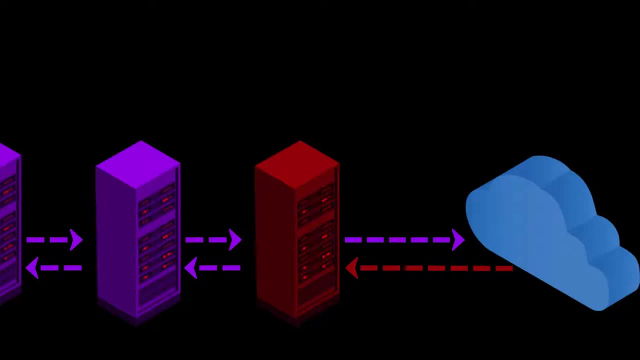 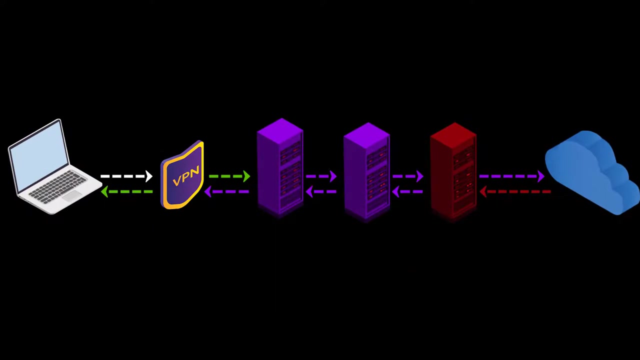 have an SSL certificate. In other words, it isn't a disadvantage of using VPN. I have just added it to this advantage list to indicate that visiting non-HTTPS addresses with only VPN used can also compromise your privacy. The only solution to this situation is to visit websites that use an SSL certificate. 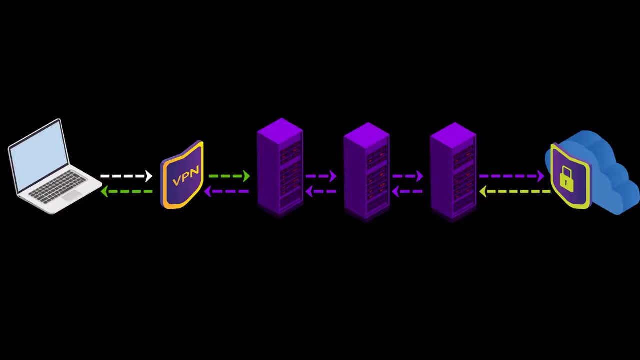 Another disadvantage is that, in addition to the slowness of the Tor network, using a VPN will slow the internet speed more. However, considering the security it brings, this is not a big loss. The priorities you should be aware of the when and how to use the VPN are the following: First of all, you should be aware of the 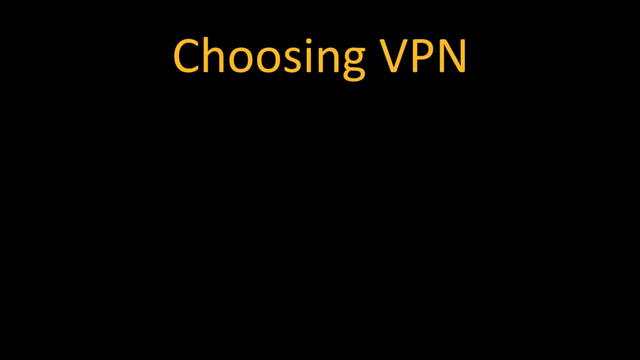 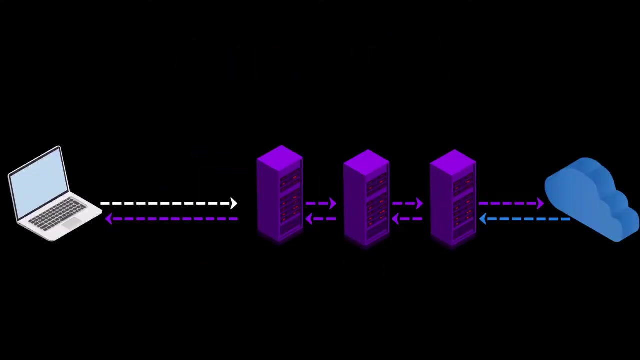 using the Tor network over VPN. It is to prefer VPN services that provide uninterrupted service, never keep logs and can payments anonymously. If you ask why these are important, If your VPN connections drop when you connections to the Tor network over VPN, observers on your network can learn that you are. 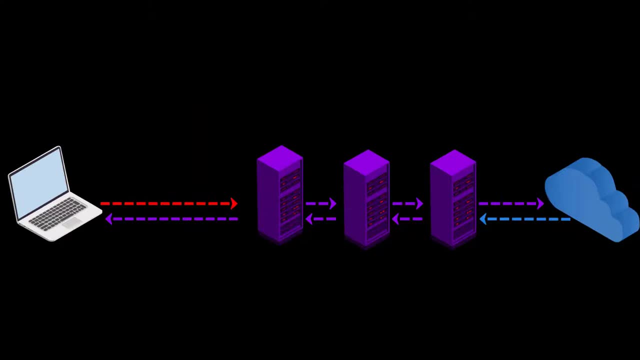 connecting to the Tor network. In addition, the entry nodes, which is the first node, can learn your real IP address During the connection drops. if the VPN service keep logs, all the security and privacy measures you take will be in vain, As the origin point of all activities. 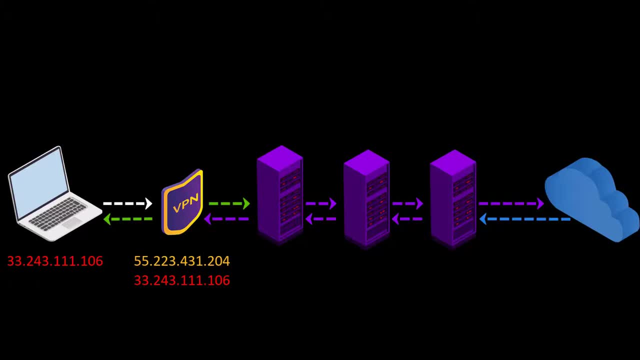 you do will be known by your VPN servers. Logging means that your entire internet record in associated with your identify. In such a case, it doesn't make much sense to be using the Tor network. When paying for a VPN service, you need to pay in cryptocurrencies to protect your holistic anonymity. Those when the IP 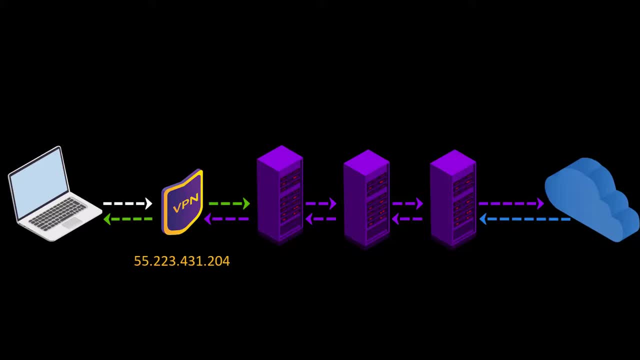 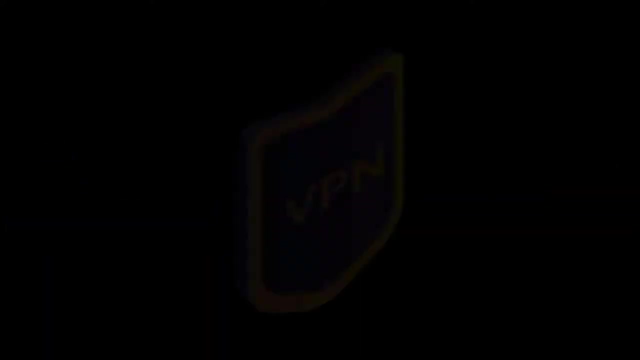 address of the VPN service. standing in front of your real IP addresses is surged. It cannot be directly associated with your real identify. In course, we will also be talking about how cryptocurrencies give us anonymity. At this point, you have to decide for yourself which is the most important. 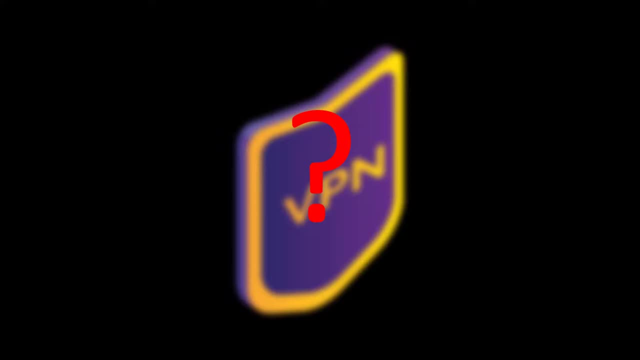 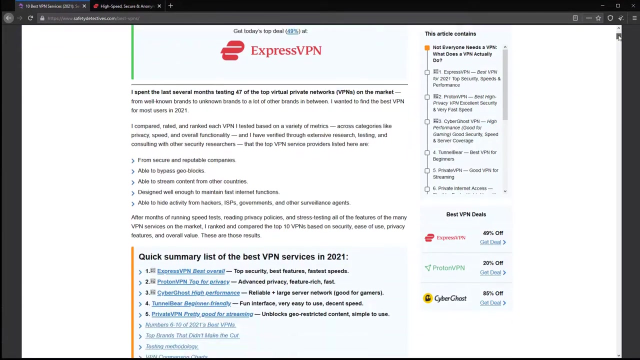 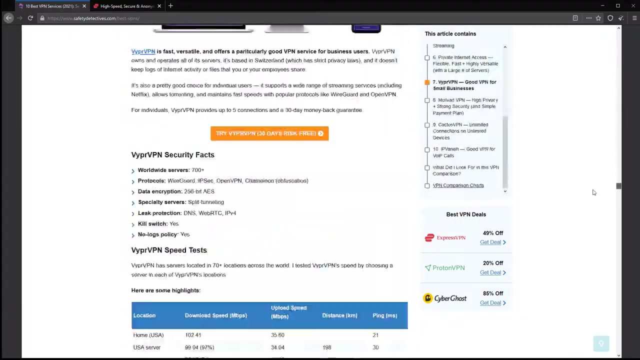 and the most ideal VPN service. It can be difficult to determine which VPN service is trusted, So you may want to check out this VPN comparison chart by the One Privacy site, which analyzes almost 200 VPN providers based on their jurisdictions and policies, For example, in the period I reviewed the list. 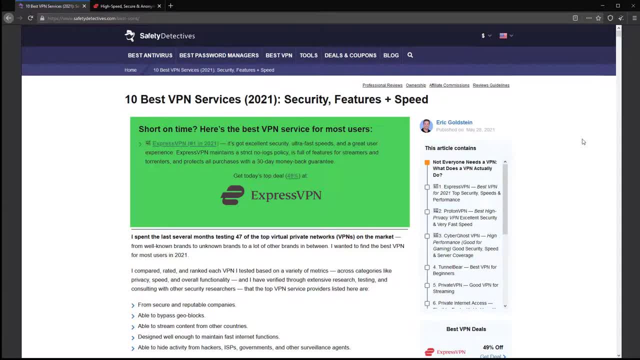 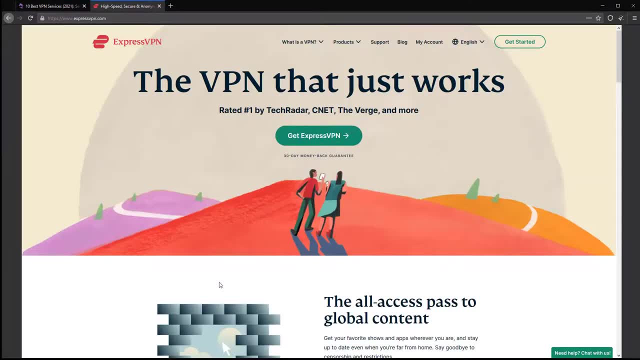 ExpressVPN was chosen as the most ideal VPN service. In addition to being on the list, according my personal experience, I can recommend you to use ExpressVPN. My recommendation reason: it has proven by independent organization that it doesn't keep logs and prevents the leak of your real IP address by 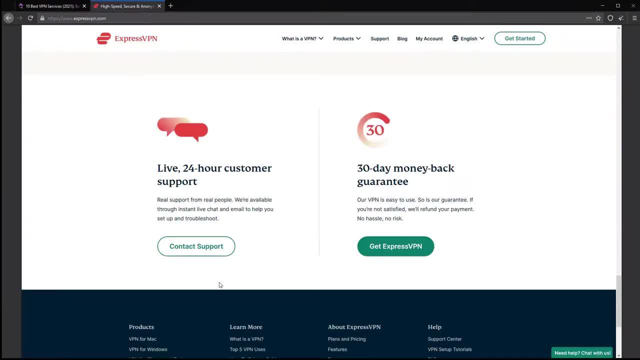 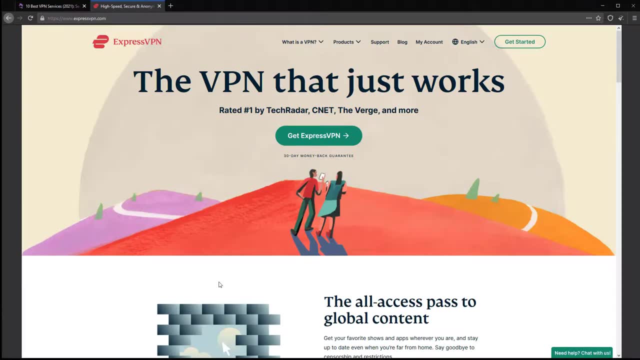 disconnecting the internet as soon as the VPN connection is lost. You can use the Bitcoin for payments and you can also get a refund if you are not satisfied by trying the service for a month. Although this service is ideal in my opinion, you can, of course, 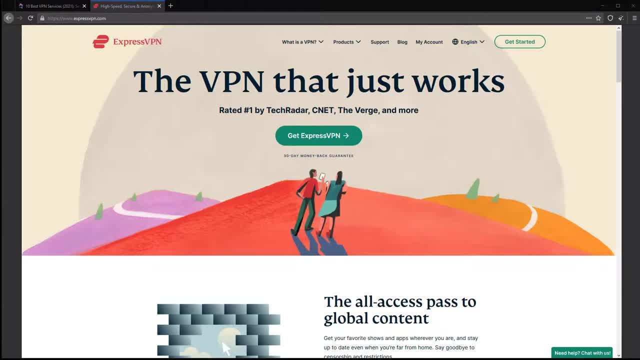 take a look at alternative services and make your own decision. In addition, what I explain here isn't an advertisement for the service. It is a service that I have specified to share my personal opinion. for suggestions purposes, I've created a special discount link for this course so that only those who want to 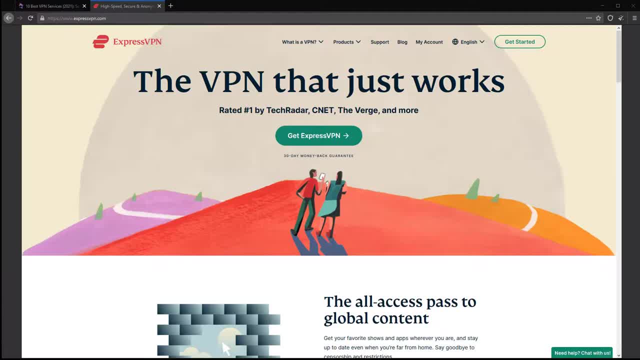 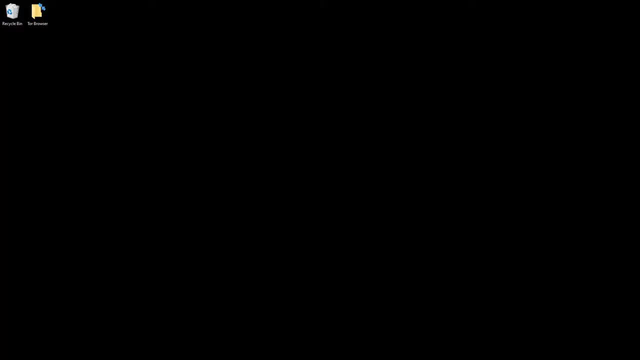 use it can use it at a discount. I have added the link to resources for this lecture. You can try it if you want to use it. After choosing right VPN service, all you have to do use Tor over VPN is to start the VPN services of your choice. 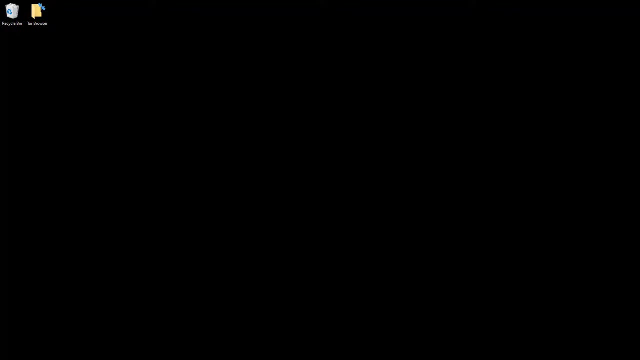 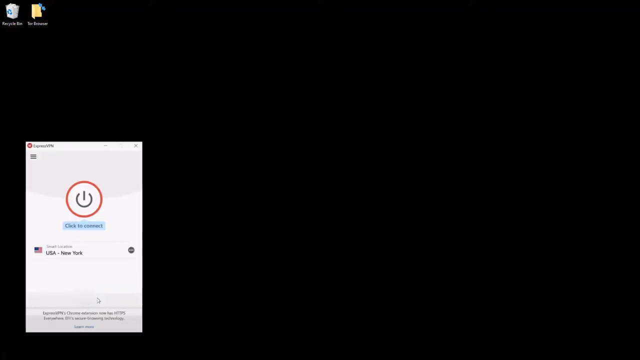 before connecting to the Tor network, To connecting to the VPN service, you need to download and install the application of your preferred service on your system. After the installation process, you can make the VPN connection very easily. For example, after establishing the VPN. 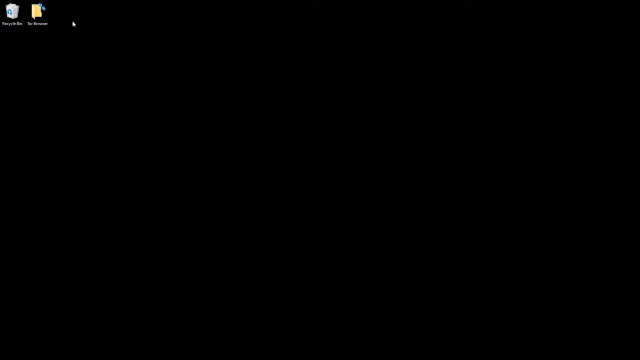 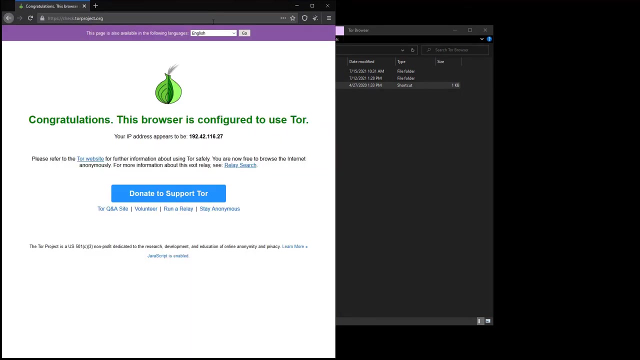 connection of the ExpressVPN service. when you connect to the Tor network through the Tor browser application, you can ensure security communication, as anyone who observes your internet and Tor network can only see that you are establishing a VPN connection.